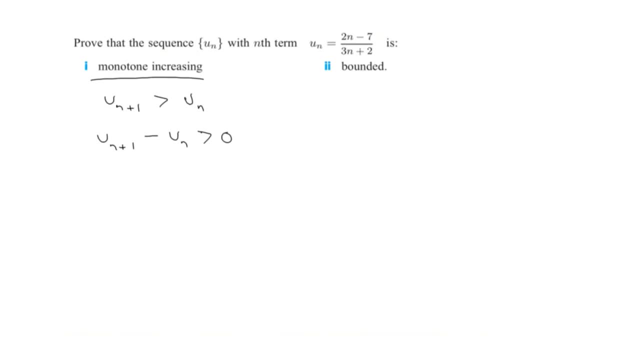 we could do. you could write the sequence as a function, as in replace the ends with x's, So in this case we might call it 2x minus 7 over 3x plus 2.. And then you could show that say f of x. 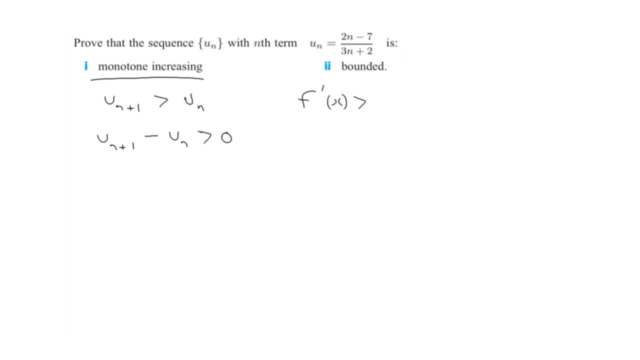 put f dashed x in, you could show that that is positive over the whole of the domain, the domain for a sequence, a natural domain, being all positive integers. So if you show that that is true, then that conclusively proves that the sequence is monotone increasing. You could if you had 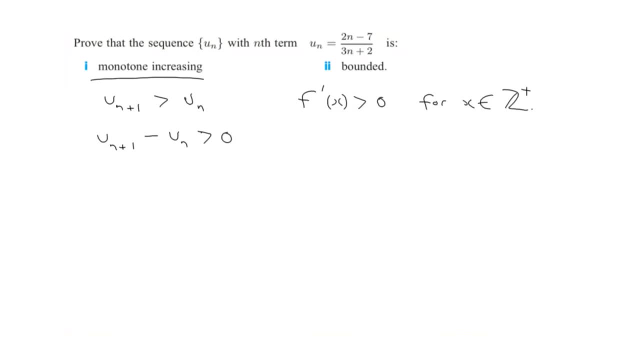 something that looked geometric, eg if it looks like to get from the current term to the next term, you multiply it by something, by a common ratio. If you can show that that ratio is well, the absolute value is greater than 1, and then it would depend on the signs. 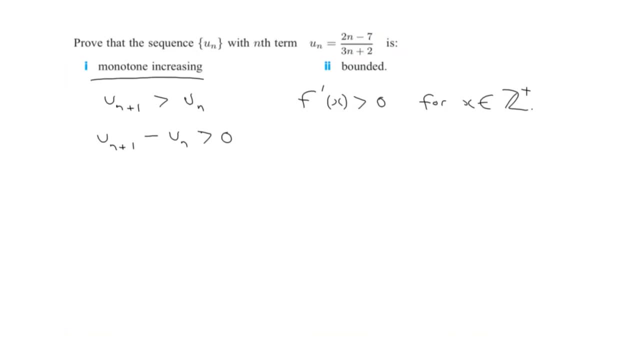 the sign of the first term and the sign of the ratio. you might be able to use that to show that it's monotone, increasing, but you definitely can't use it for this because it's not geometric. So for this to be honest, using the derivative or using 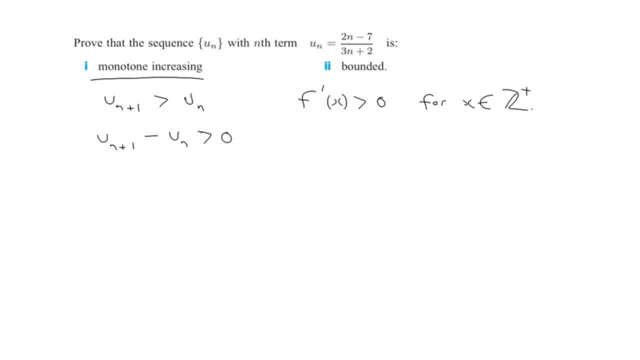 this: un plus one minus un. I think probably the amount of work involved is similar, but I am going to use this first method. So we're going to get an expression for the next term minus the current term. So the next term, well it's, if the nth term is two, n minus seven, over three, n plus two, then 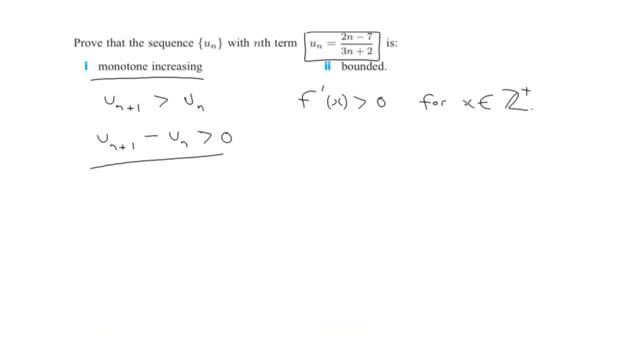 the n plus one term. we just replace n with n plus one. make sure you use brackets. so um u n plus one minus un. well, that is going to equal: it's two n plus one minus seven over three n plus one plus two. so that's the n plus one term. subtract the nth term which is just given to us. 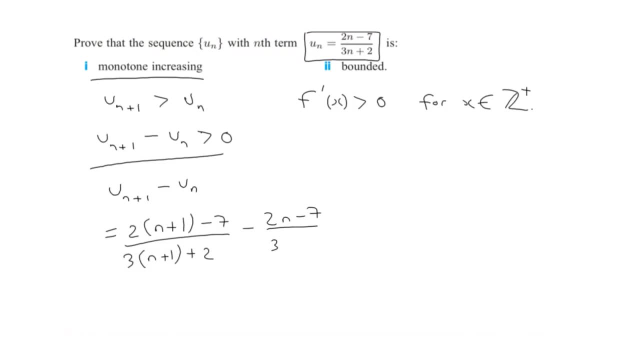 minus two, n minus seven, over three n plus two and something like that. I'm going to have to do quite a lot of tidying up for this. so the first thing we're going to look at is this, this first term. so let's get rid of those brackets. So two n plus one minus seven is going to be two n plus two. 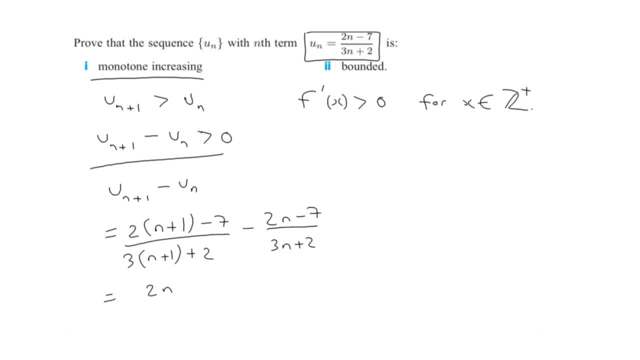 minus seven, which is two n minus five, two n minus five, and the denominator three n three brackets n plus one is three n plus three. plus the two must be three n plus five, and then minus two n minus seven over three n plus two. So now, if we look at that, remember I'm all I'm looking to do. 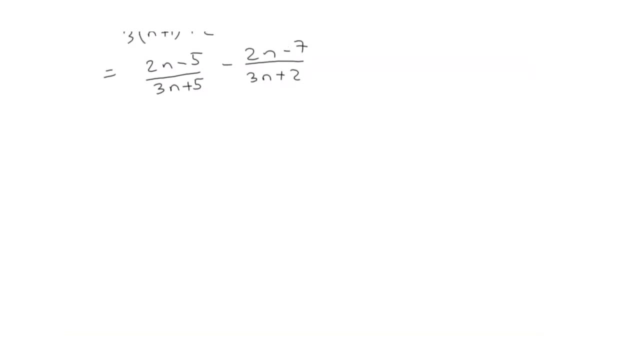 is show that this is always positive for monotone increasing. so what I am going to do, I have one expression for this and there's no friendly common denominator that jumps out at you, so, sadly, you're going to have to to cross, multiply to find the denominator. so it's going to be three n plus two. 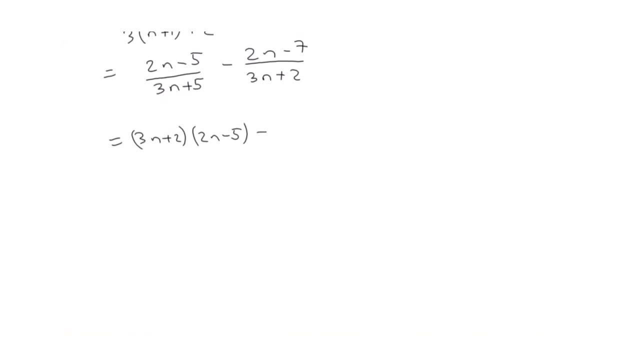 two n minus five minus three n plus five, two n minus seven, all over three n plus five and three n plus two. so we are definitely going to expand the numerator. there's no advantage in expanding the denominator, remember. all we need to do is show that this thing is always positive. so actually, if you think about the denominator, 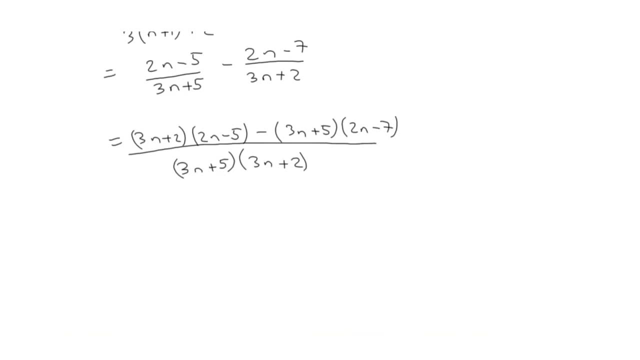 look at the denominator. there's enough there anyway. I'll discuss that in a bit more detail. but you can see on the bottom of this thing there is enough information to say that the denominator will always be positive for positive integer n. okay, so on the top you're. 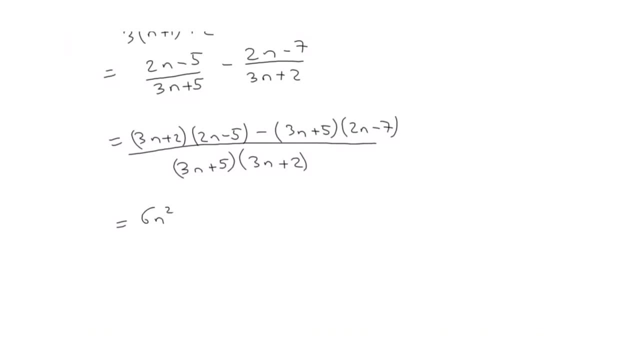 going to have all three n times two, right. so six n squared. three n times minus five, minus fifteen n. two n times two is four plus four n, so that's minus eleven n. two times minus five is minus ten. that's not forget the bracket. three n times two n is six n squared, and you've got three n times. 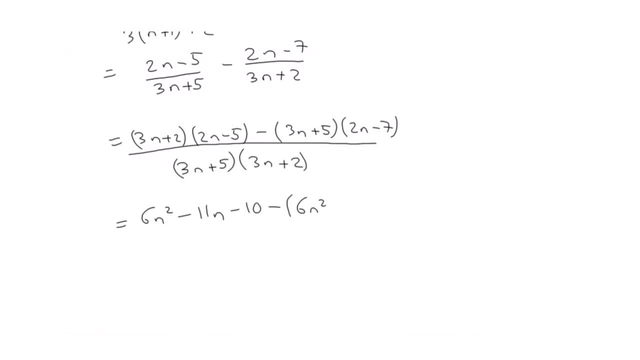 minus seven is minus twenty one n. five times two n is plus ten n. so minus twenty one plus ten is minus eleven n and you've got five. sevens of thirty five is up to be minus thirty five. so this is going to simplify it nicely over three n plus five. 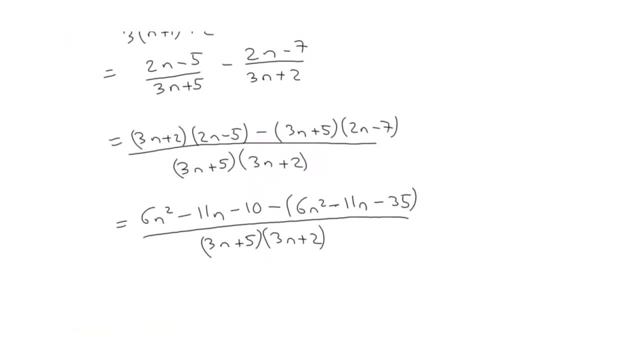 three n plus two. so looking at the top, because of this bracket you've got six n squared minus six n squared, so that's just going to be nothing. same case with the minus eleven n. so minus eleven n, minus minus eleven n will just get us to zero as well. so you've got minus ten. 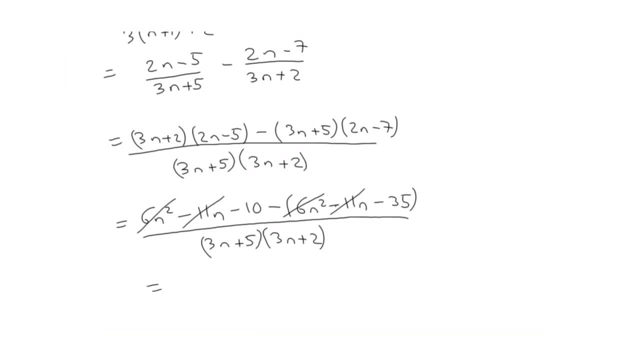 minus minus thirty five, which is twenty five. so now this equals twenty five over three, n plus five over three n plus two. now, remember, n is a positive integer, so twenty five is obviously positive. so this is positive over well. for positive integer n, well, three n will be. 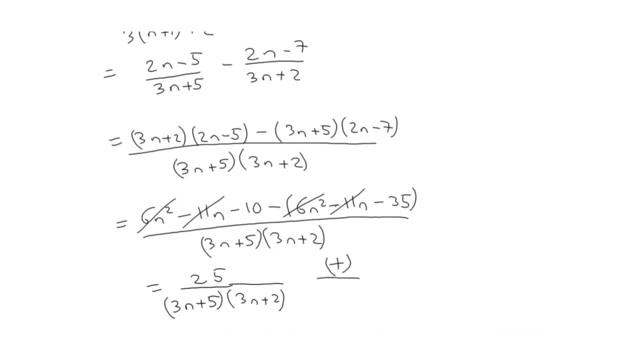 positive three n plus five will be positive. very similar argument for the three n plus two. so you're going to have another positive times, a positive on the bottom. so that means that's u n plus one minus u n is always greater than zero for a positive integer n and that means that 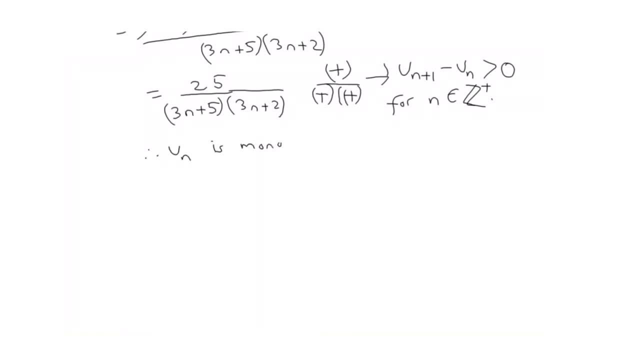 u n is monotone, increasing, or it's monotonic and it's monotonic increasing. remember, monotonic means it's either increasing or decreasing over the whole of its domain, and obviously then we just say: well, which one is it? so the second part of the question: 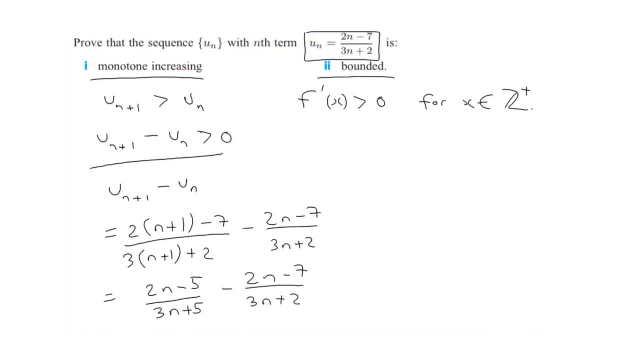 we need to show that this is bounded. so we need to show that u n equals 2 n minus 7 over 3 n plus 2 is bounded. so, basically, because this part 2 as u n, is monotone, increasing, so u 1 must be the smallest term, u 1 must be. 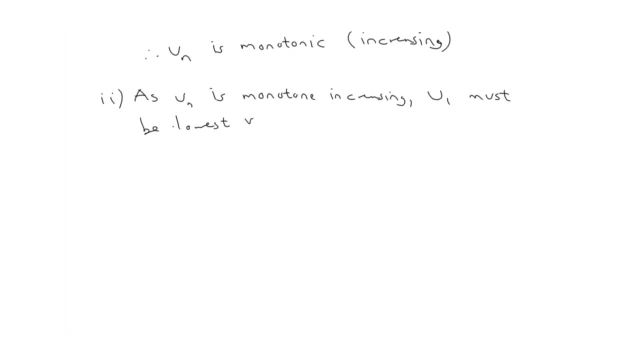 the lowest term value, eg the lower bound. So it is 2 times 1 minus 7 over 3 times 1 plus 2.. So u1 equals 2 times 1 minus 7 over 3 times 1 plus 2.. 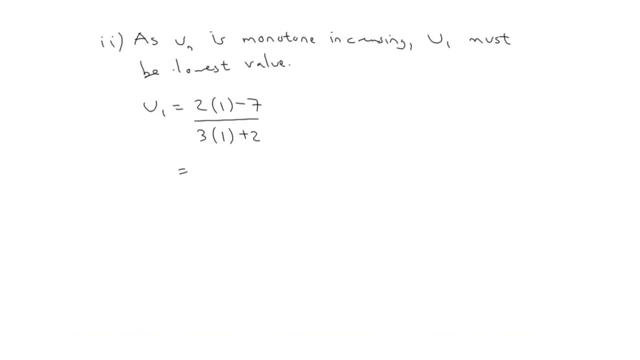 So that is: or 2 minus 7 is minus 5, 3 plus 2 is 5, so minus 5 over 5 equals minus 1.. So lower bound, lower bound, is minus 1.. Now for the upper bound. again you've got. 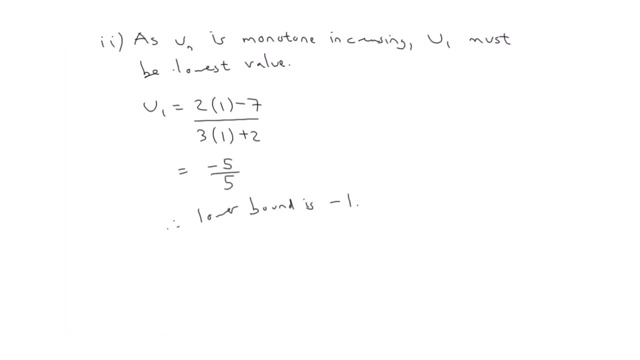 options. There's kind of a quicker, or it could be argued that it's quicker and possibly easier, depending on what you're trying to find. You could get a bound that's not really anywhere near the actual upper bound, but it does show that it's bounded, So I'll show that first. So basically, u1. 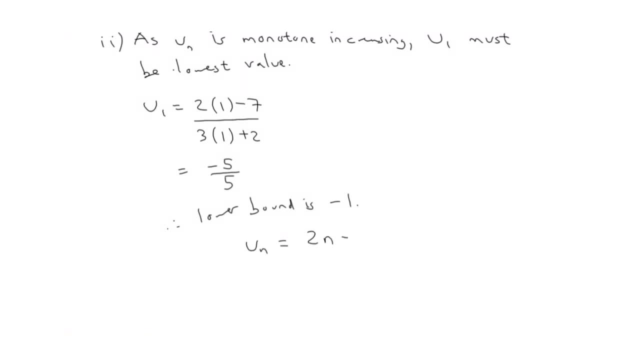 equals 2n minus 7 over 3n plus 2.. So basically, we can very quickly show that this will never get beyond 1, if you think about it. So for the n's that we're interested in, which are positive integer n's: 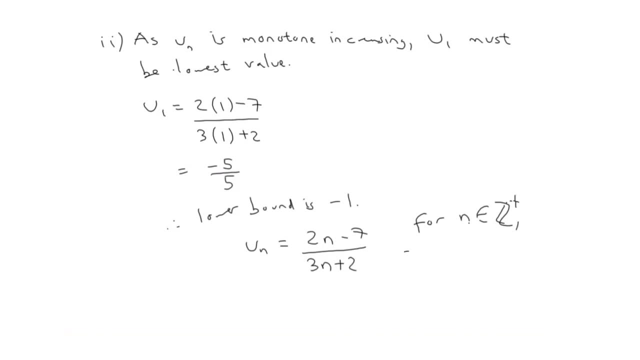 for positive integer n's 2n is always going to be less than 3n and the minus 7 is going to be always less than 2.. So the reason why we pick those is because you've got the 3n here and the 2. 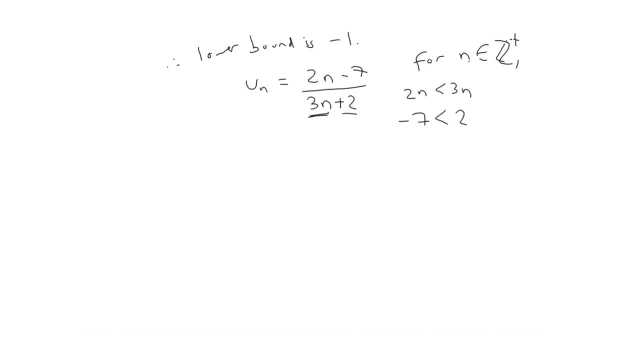 here. So if 2n is always less than 3n and the minus 7 is always less than 2, so 2n minus 7 over 3n plus 2 is always going to be less than 3n plus 2. 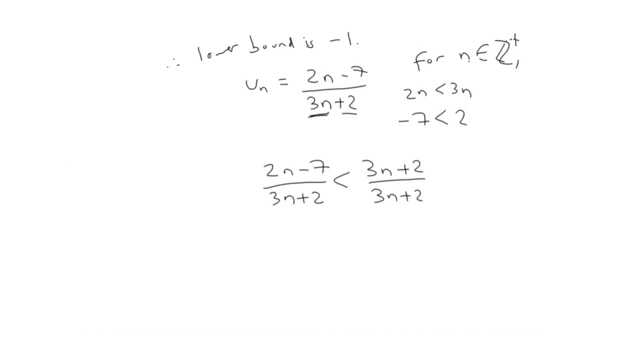 over 3n plus 2, because obviously the smaller the value of the numerator will make the whole thing smaller. So 3n plus 2 over 3n minus 2.. So 3n plus 2 over 3n plus 2 is obviously 1..